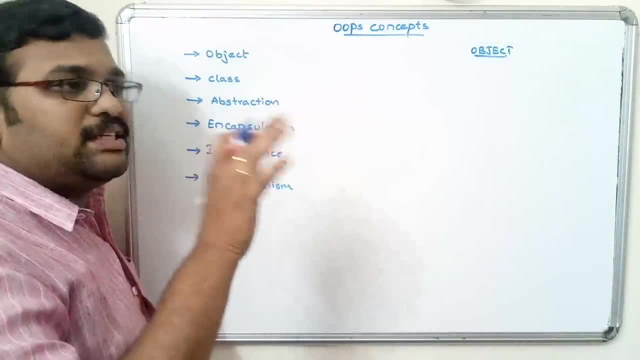 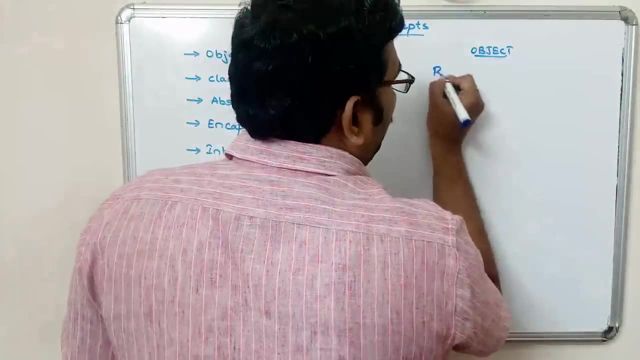 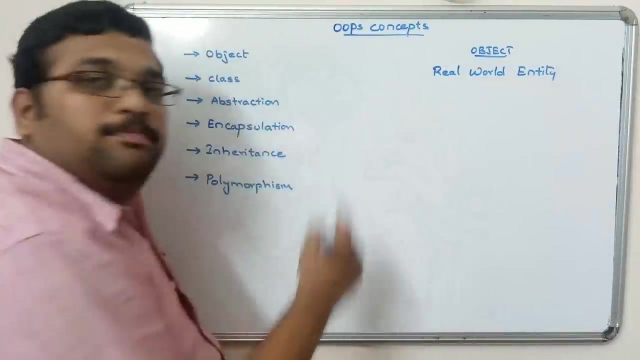 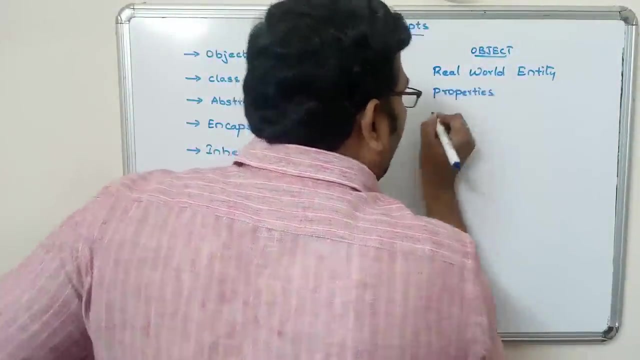 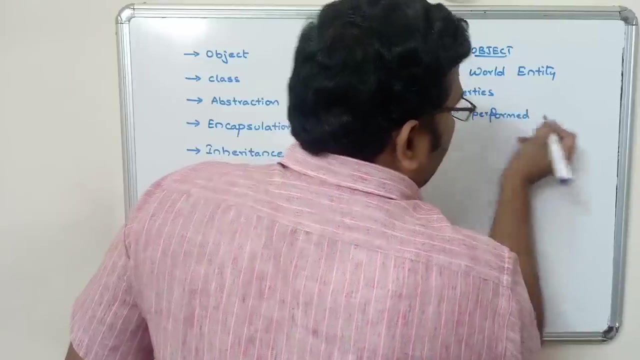 world entity. so whatever the thing we are seeing in the real world that can be treated as an object, so this object is a real world entity and this object consists of so properties and the task performed by task performed by this object. so whatever the real world entity which is 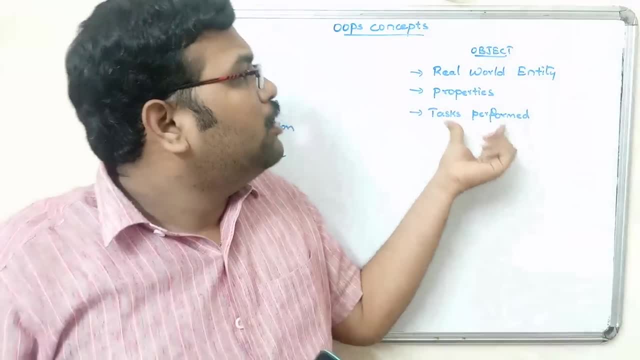 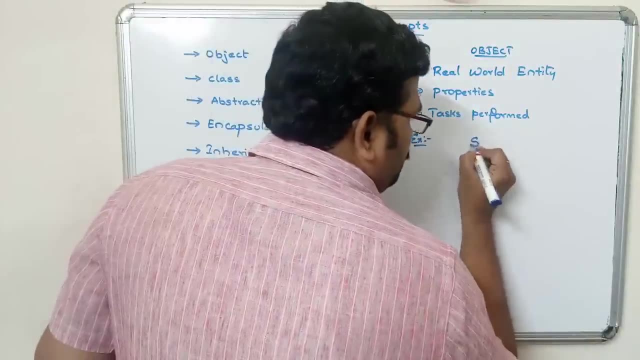 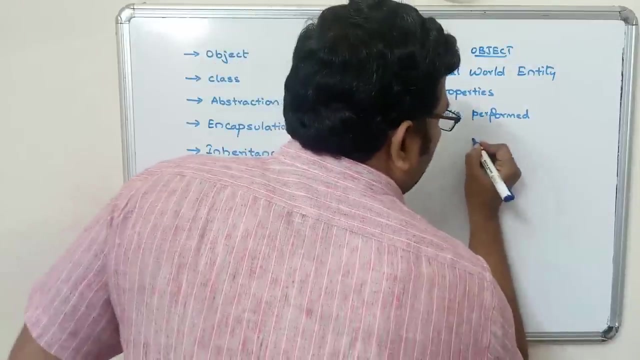 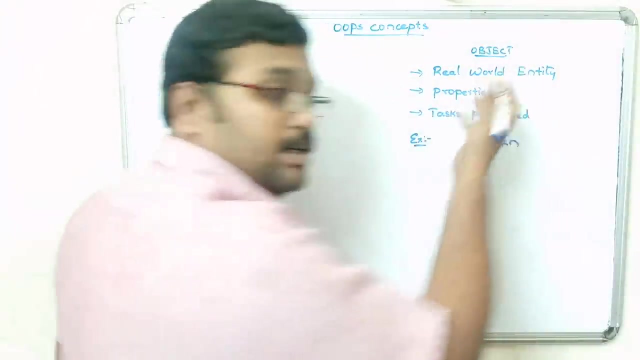 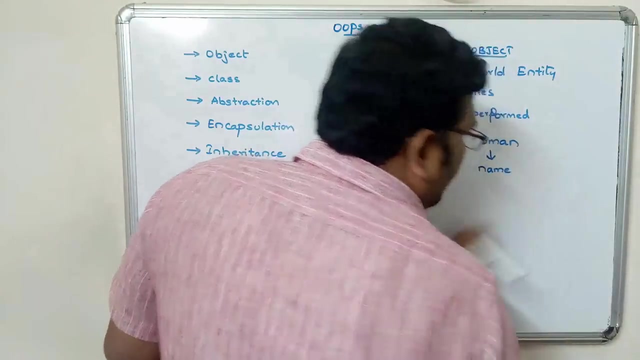 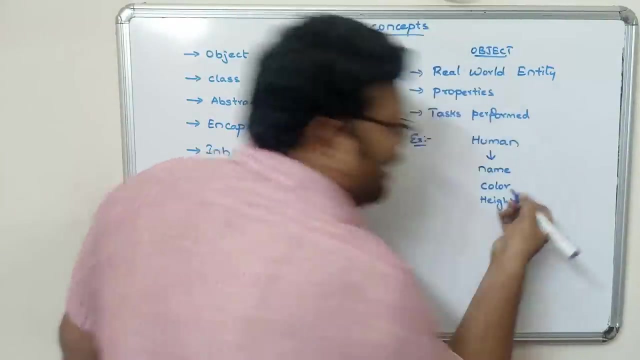 having these properties and the task, some task to be performed, those we call as a object. let us take an example: human human being is also a human being, it is also an entity, I mean, it is also an object. so human consists of properties like name, color, height and etc. so these are the properties, so what this human can do. 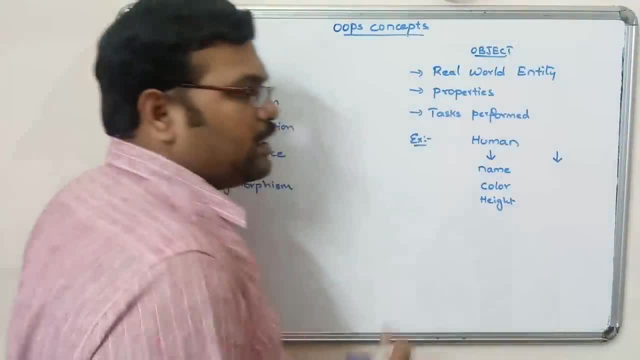 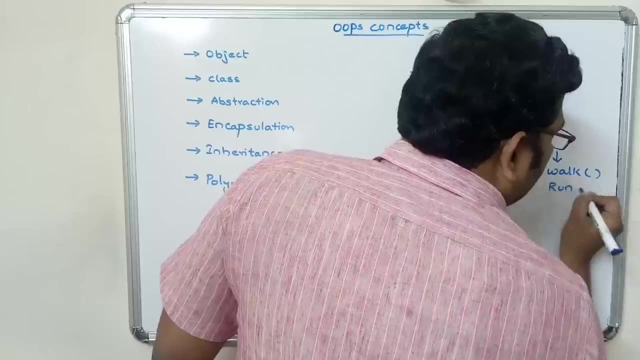 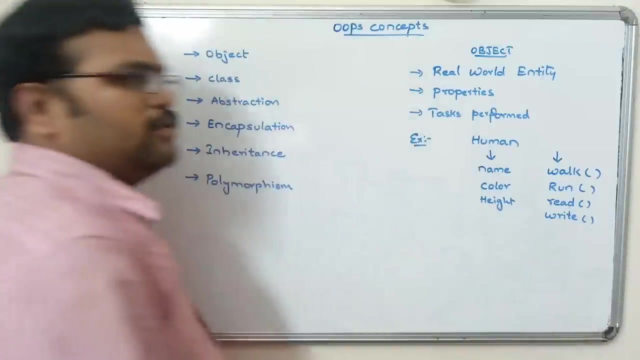 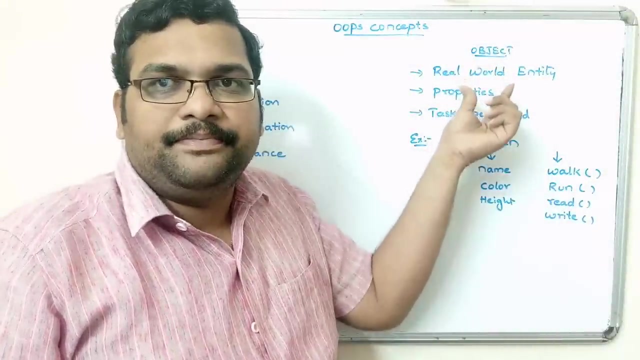 the task. what are the tasks can be done by this human: walk, run, read, write, etc. so these are the tasks can be performed by this human. so we can consider this human as a object. right, hope you understood. so object is a real world entity which is having 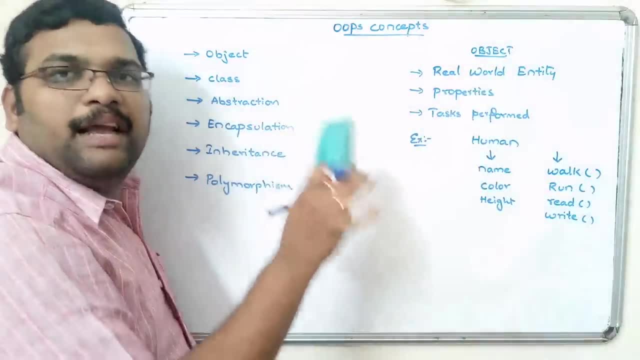 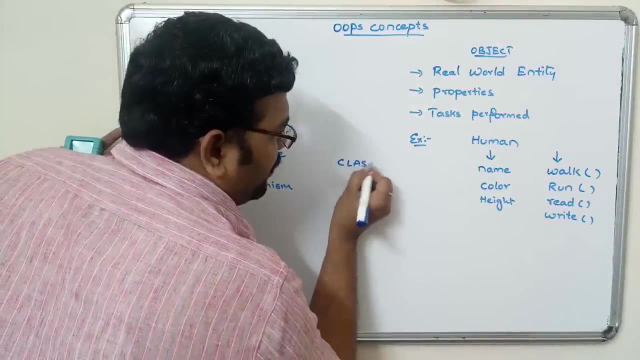 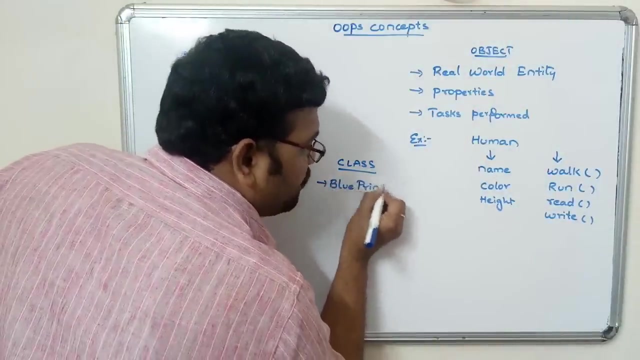 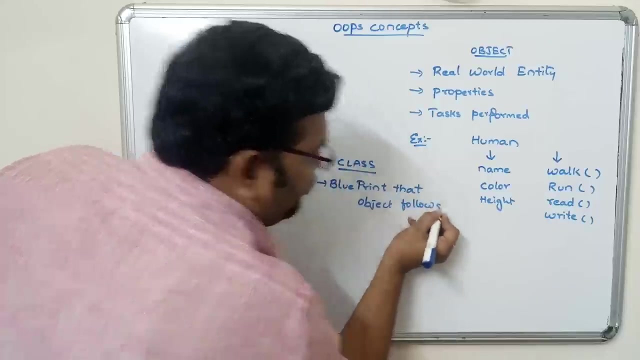 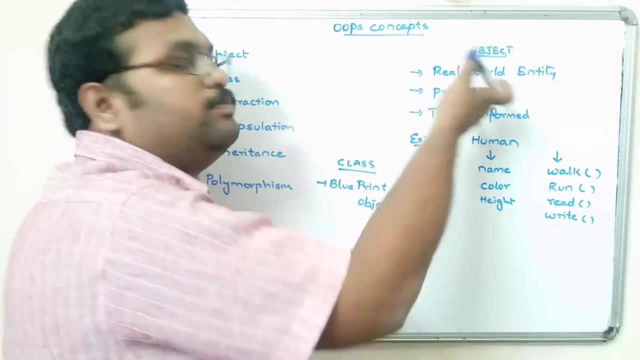 the properties and some tasks that can that it can be performed right now. what about the class? what is the class? so class is a blueprint that object follows, that object follows. so it is a blueprint that an object follows. so without the class, object is not there. so this class consist of N number. 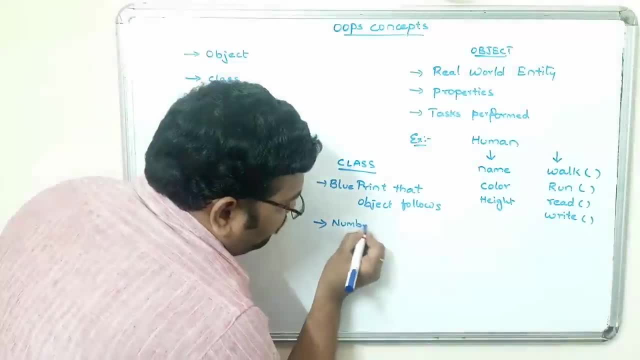 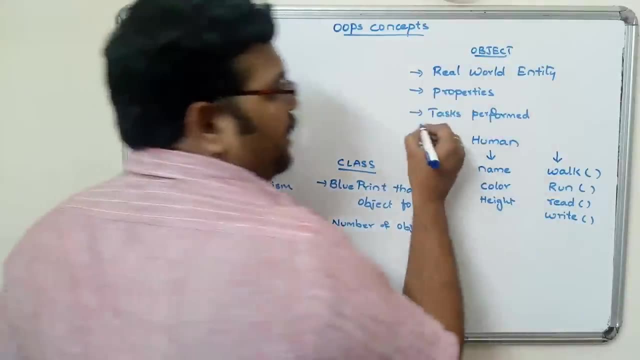 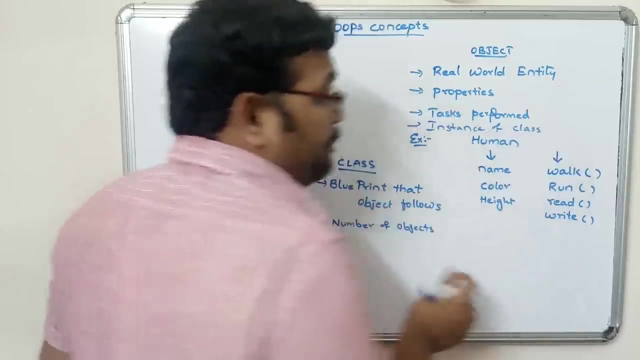 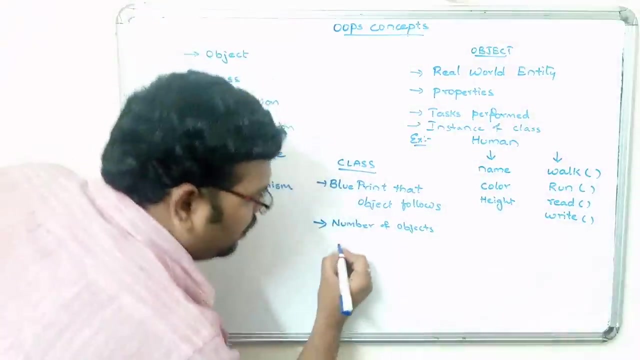 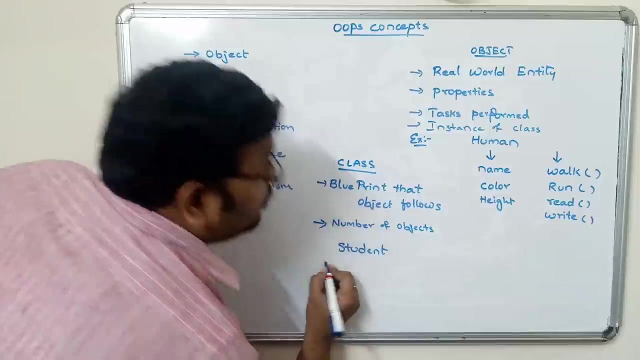 of objects. number of objects. it consists of number of objects and object can be defined as instance of a class. instance of a class, so that means object will follow the prototype defined by this class example. let us take a student: student in a class, student in a classroom. so what are the properties? so 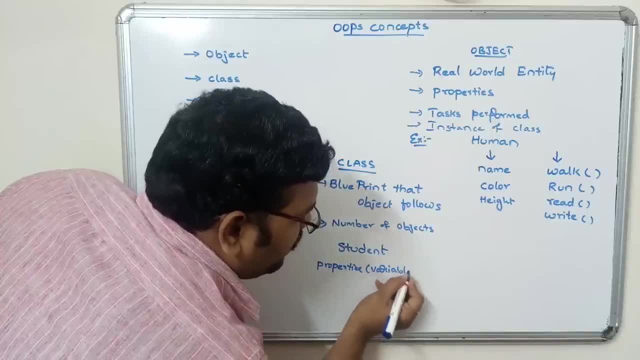 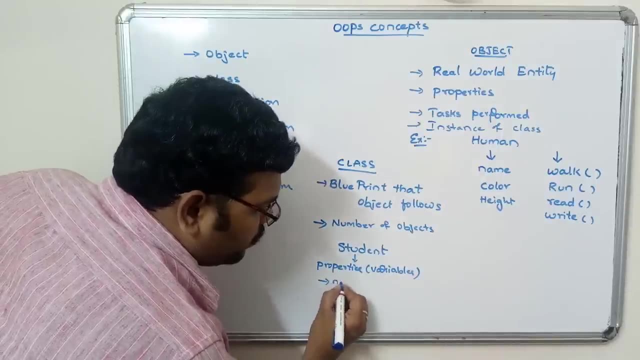 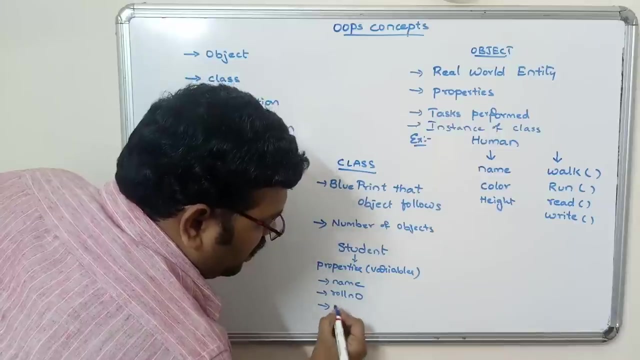 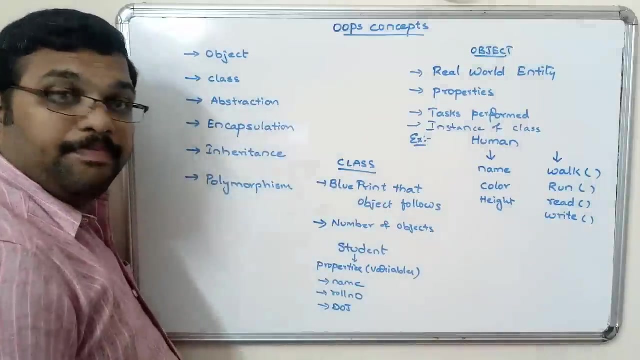 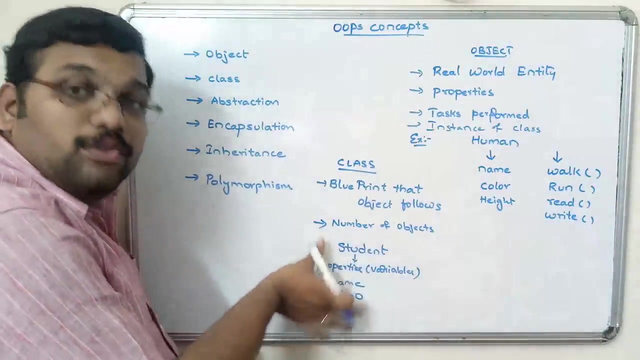 properties or variables. we can say them as a variables. so properties of a student, one student name, student roll number and student date of joining- date of join right. so this is a class and all the objects which are defined by this class should follow this prototype so that, for example, a student in a class there 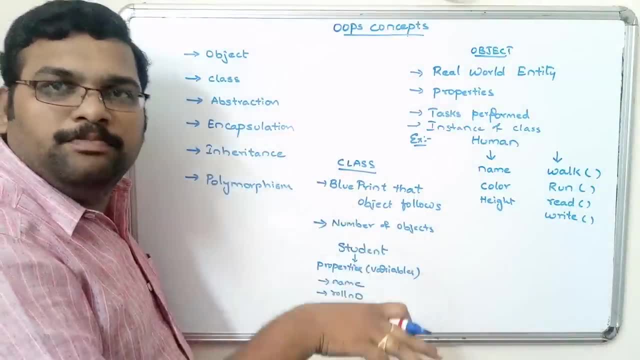 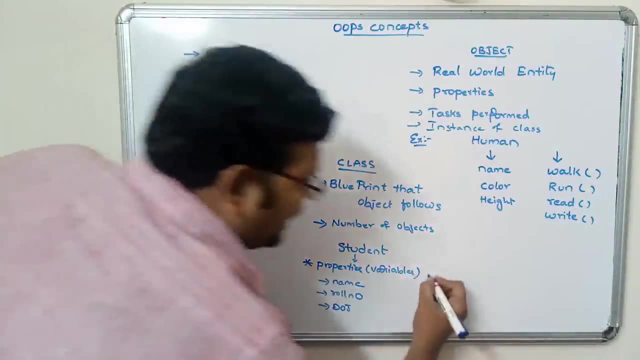 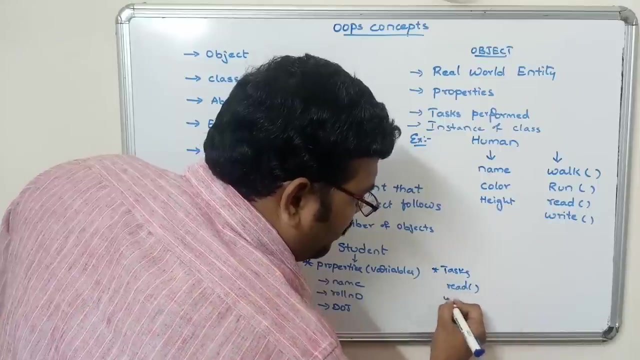 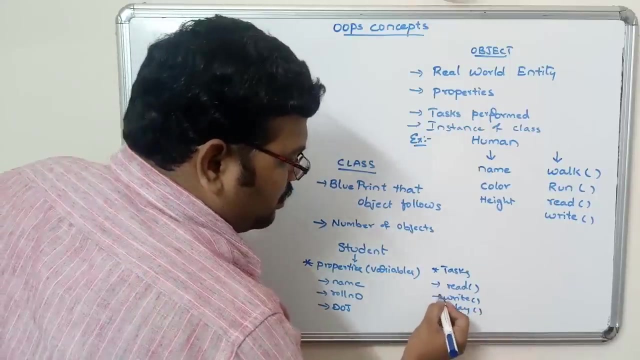 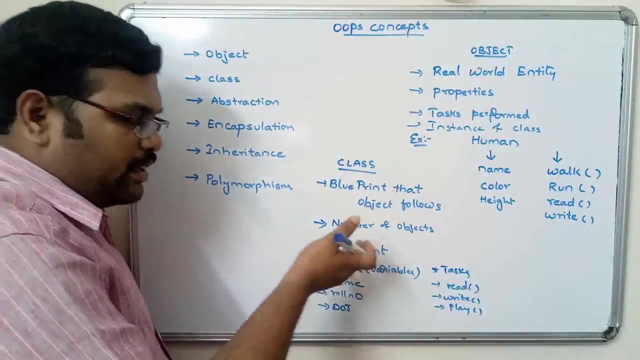 are n number of students. every student can be considered as an object which follows the same prototype and one of the tasks to be performed by the student- read, write, play, right, so every student can have three properties: read, write and play. every student will be having the three properties: name, roll number and some. 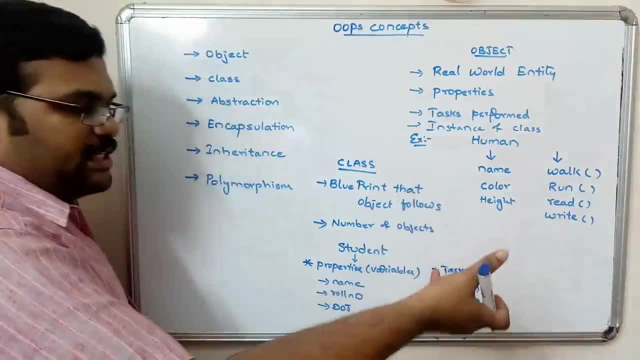 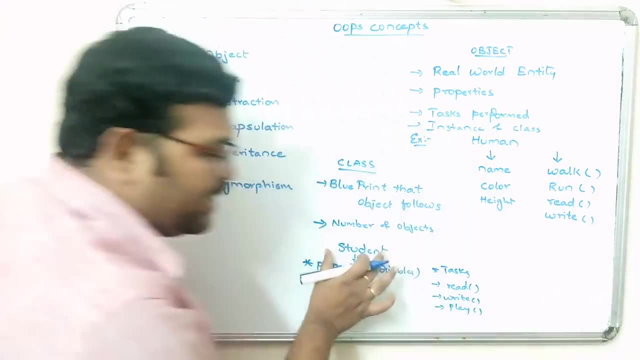 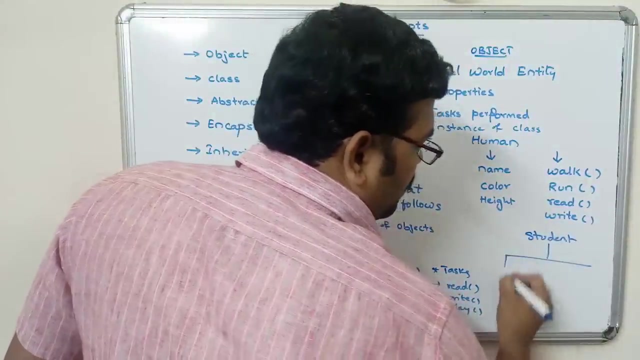 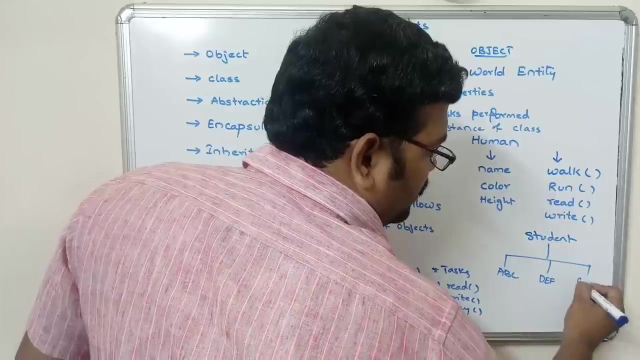 date of join. so whatever the objects created through this class will follow the same structure. that means what is the same structure: objects. so student consists of a number of objects. so student class consists of some ABC, the name of a student, ABC, some DEF, some GHI, so ABC will be having name. 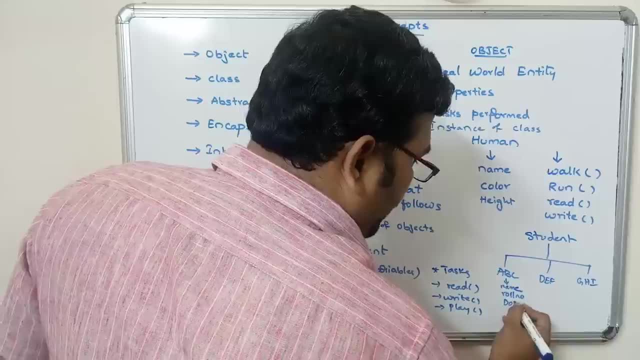 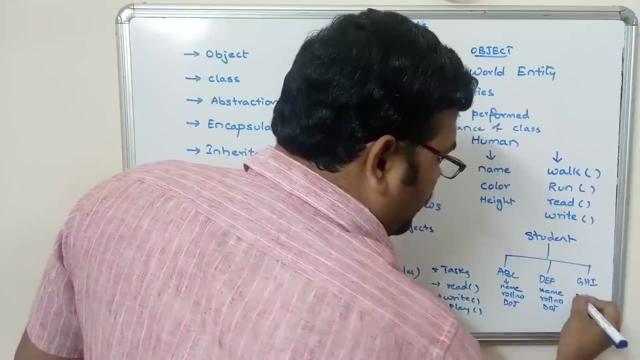 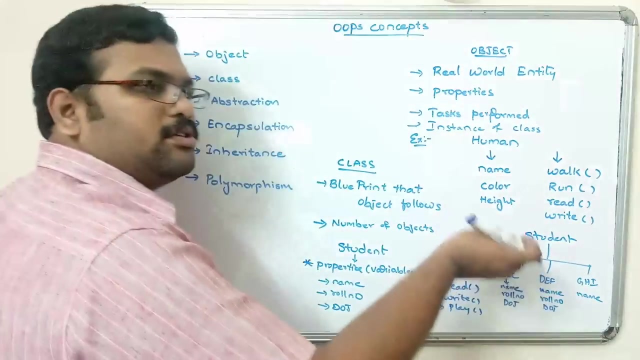 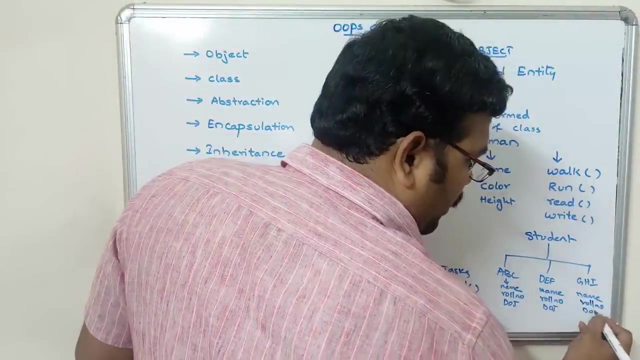 roll number: date of join: name: roll number: date of join, similarly GHI. so here ABC, DEF, GHI are the names: name of a student, let it be like Sandeep Saradi and Samsuresh. roll number and date of join and for every student. 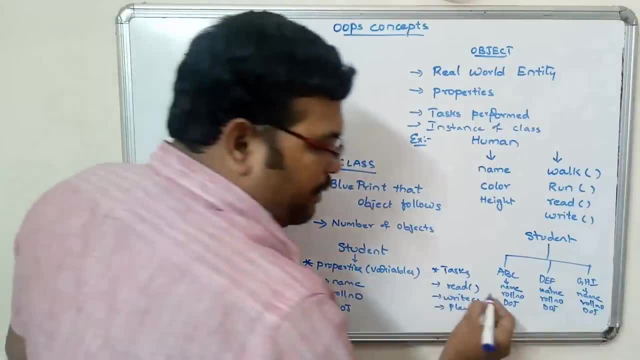 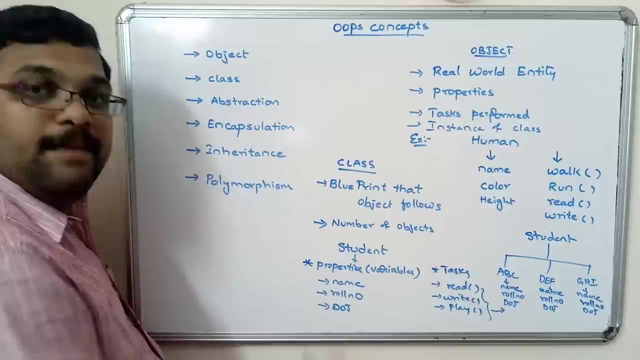 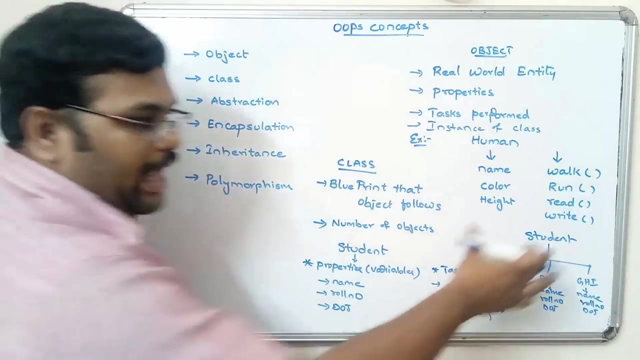 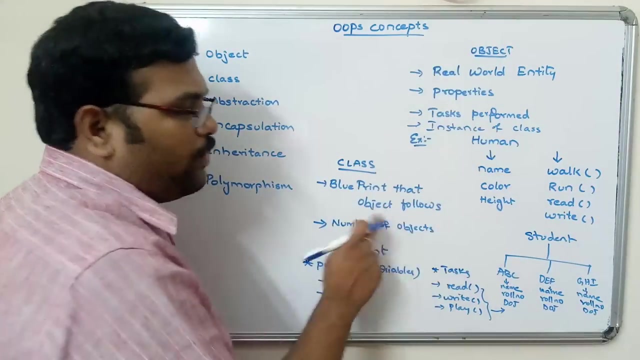 will follow some properties. some read, write and play. So these three properties can be done and be invoked by this ABC and these properties can be applied for DEF and these properties can be gone by GHI. so an object is an instance of a class and a class is a blueprint that the object should fallso a class. 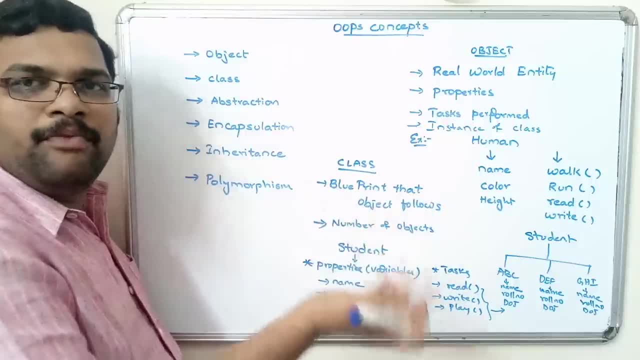 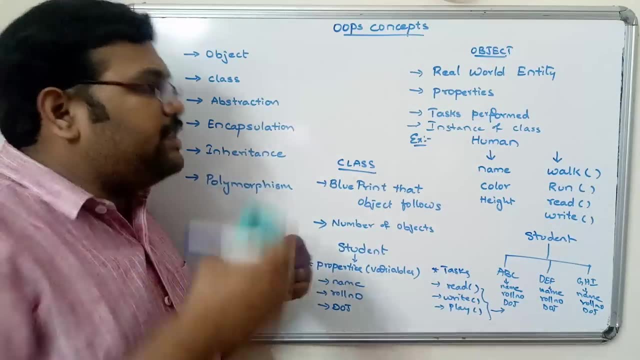 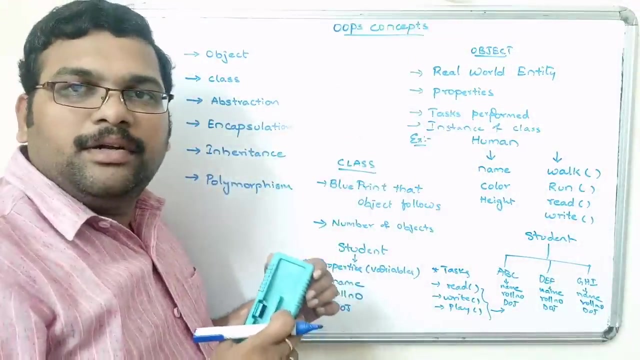 consists of n number of objects, objects, many number of objects. hope you understood this- object and class, because our java programming completely deals with these two things: class and object. for everything we will create a class and we will create an object. so a class cannot run the methods of another class directly. so one class of 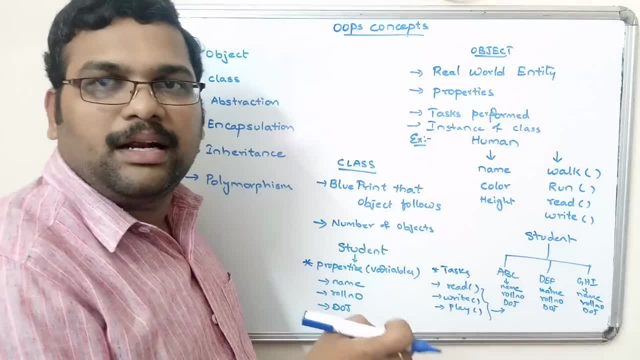 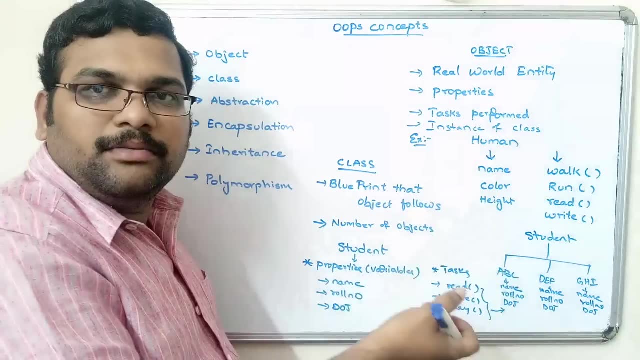 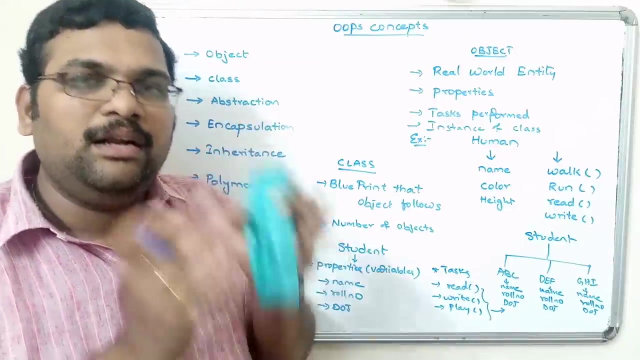 methods cannot be invoked by the another, another class. so in order to access the methods of another class, one class should create its own object. so simply we can say: a classes cannot communicate with each other, but in order to communicate with each other, object should be created. so for every. 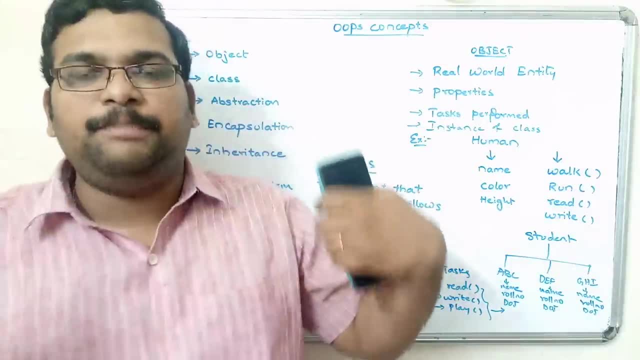 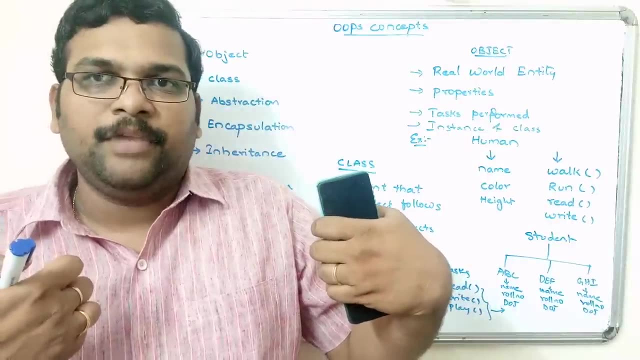 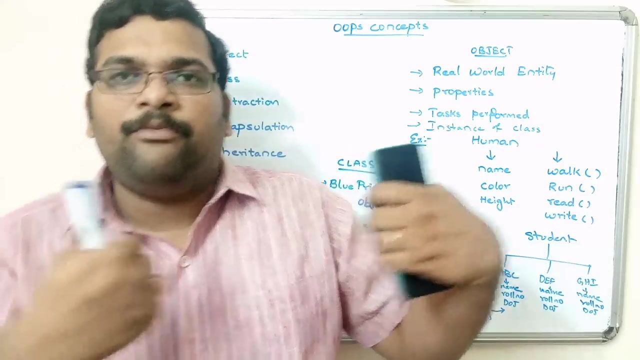 communication object should be created, so if class a and class b wants to communicate, so here the communication means invoking the methods of one class by another class. so every class is having the methods right, so tasks. so invoking those methods or tasks from one class to another class is called a communication, and this cannot be done. 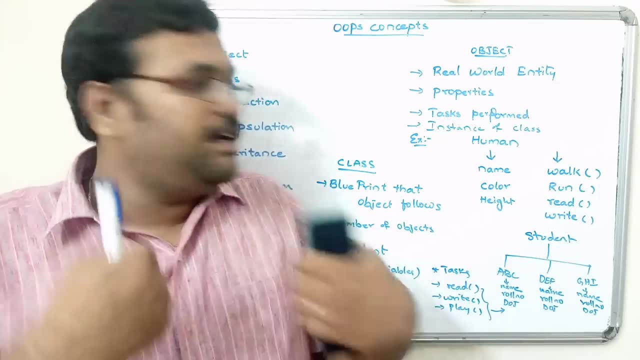 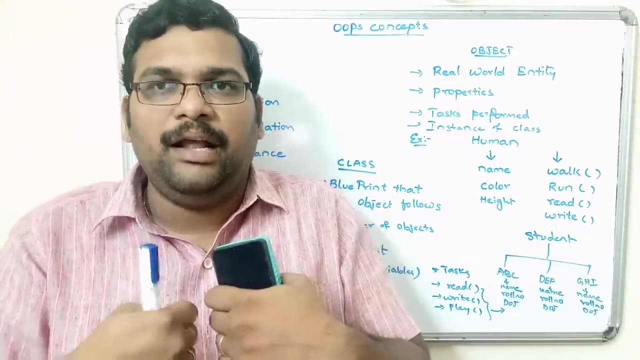 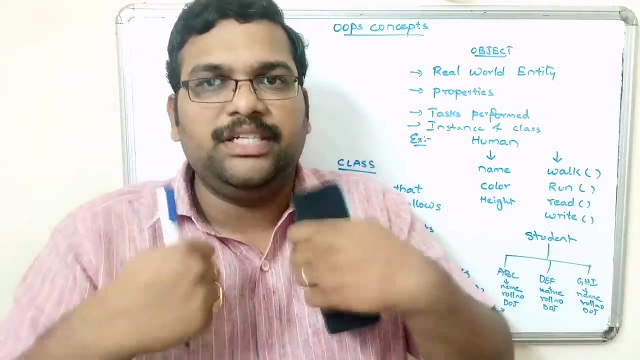 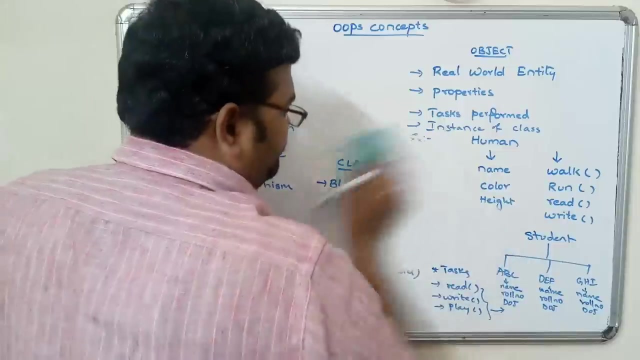 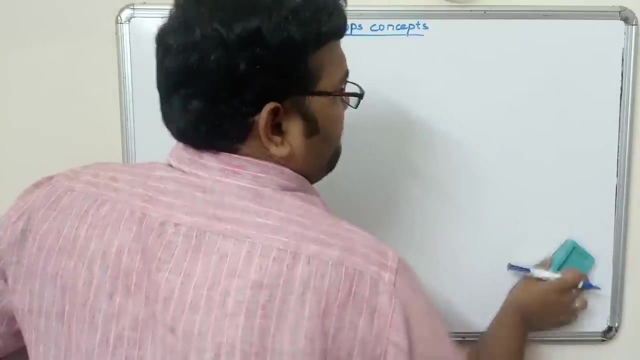 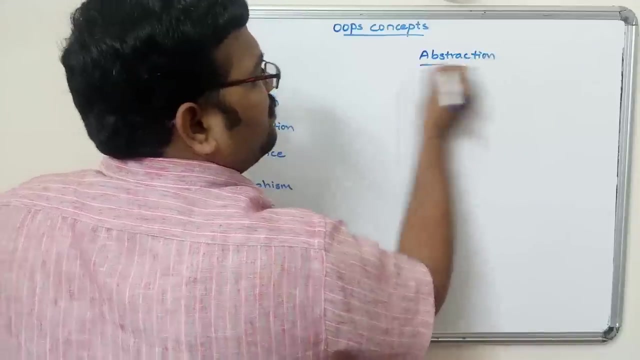 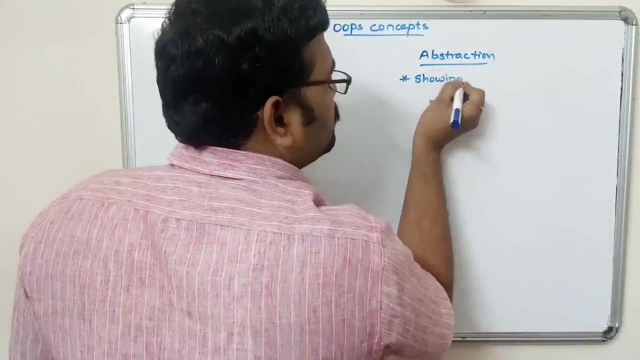 between two classes, and this can be done only between objects. so in order to communicate two classes, first their instances should be generated, and through those instances though the two classes will be communicated. so hope you understood this thing. the class and object. next, abstraction. abstraction means showing only essential parts, only essential parts. 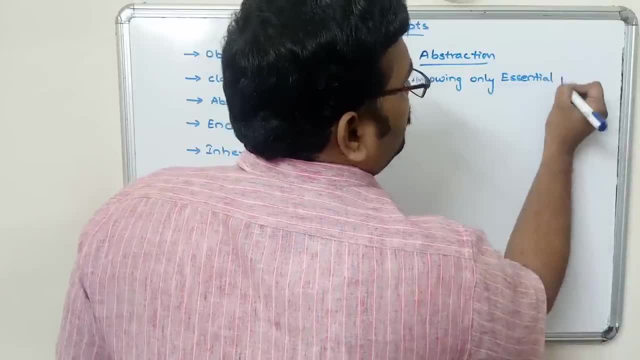 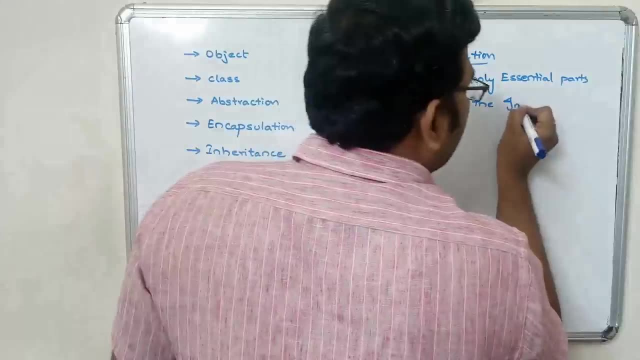 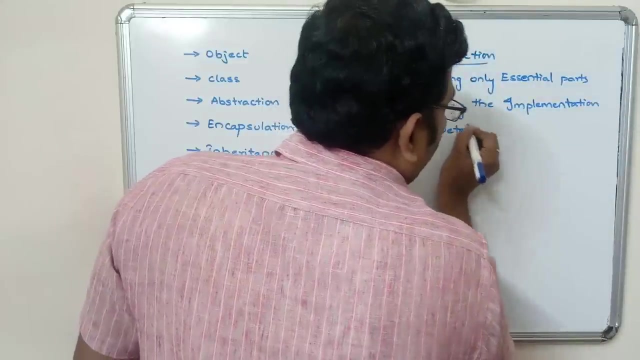 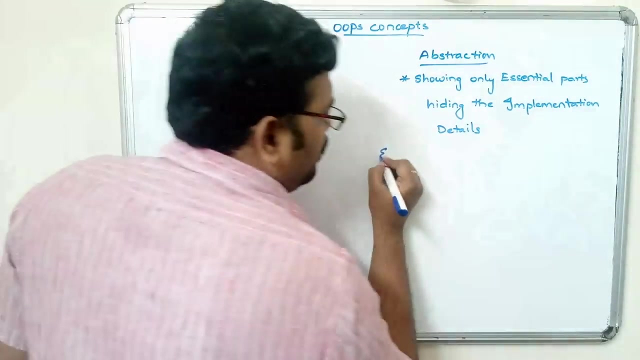 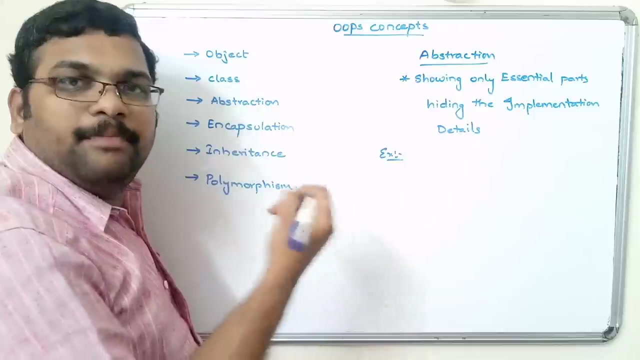 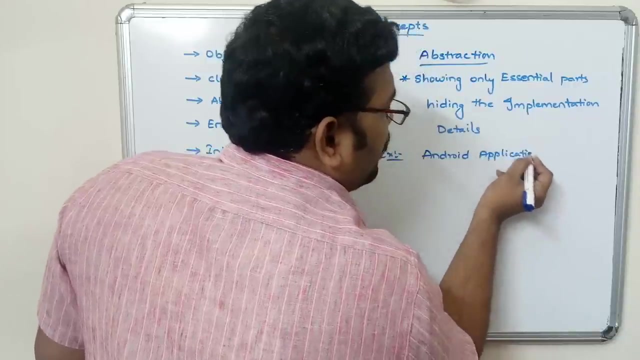 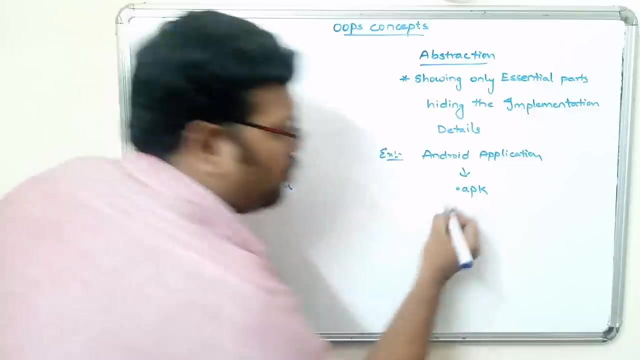 and hiding implementation details. this is called abstraction. this can be achieved in this Java programming, just the best example. so if you download an Android application from the place tool, so we will get a dot APK file, right dot APK file. or you can download a software so that we can get dot exefile. and if you 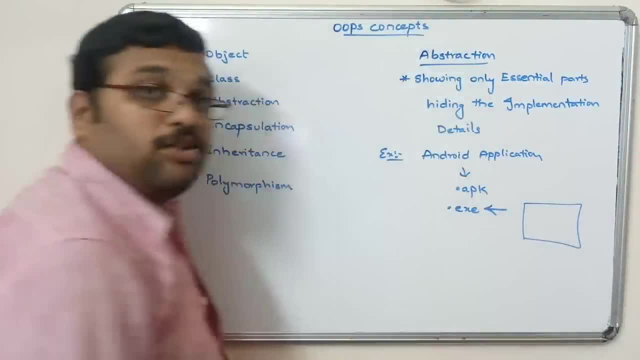 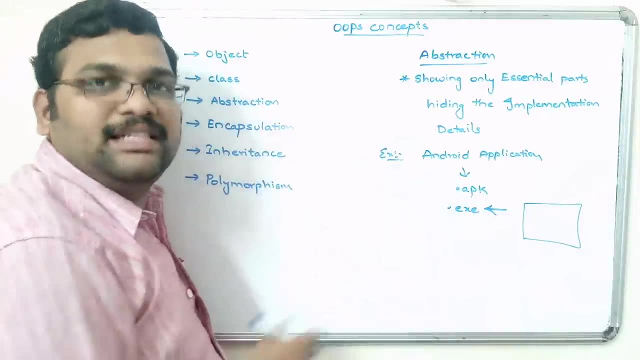 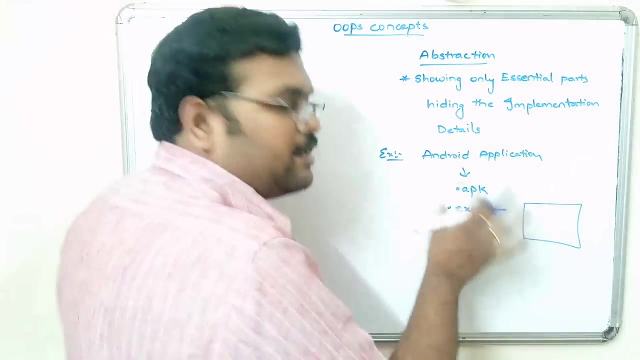 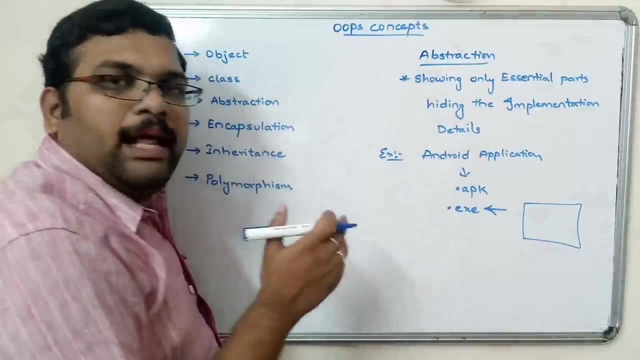 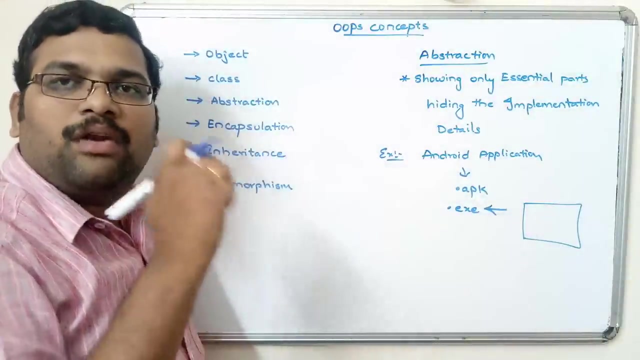 run this exefile, we can get the software and we can use the software, but here we can't see the packages or methods or functions which are used to create this exefile. that means All the implementation part is hidden and only the essential part is visible. So this is the best example. So, similarly, if you download an application from android play store, you will get a apk file, but you will not get the methods or packages or any functions which are written to generate this apk file. 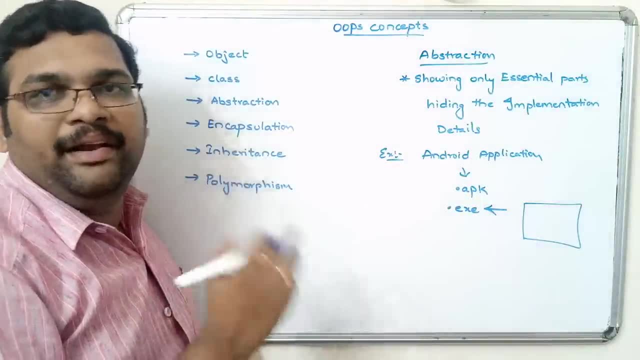 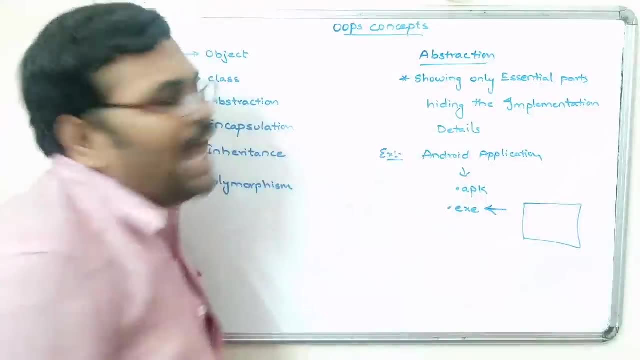 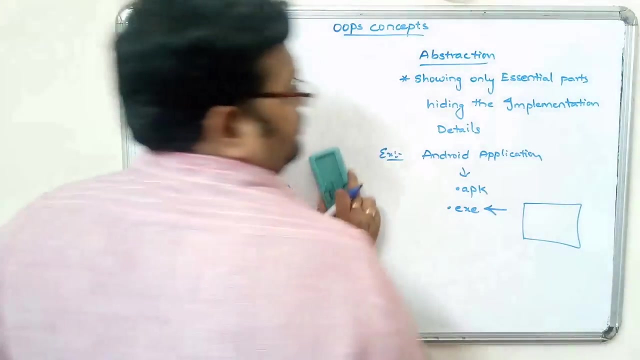 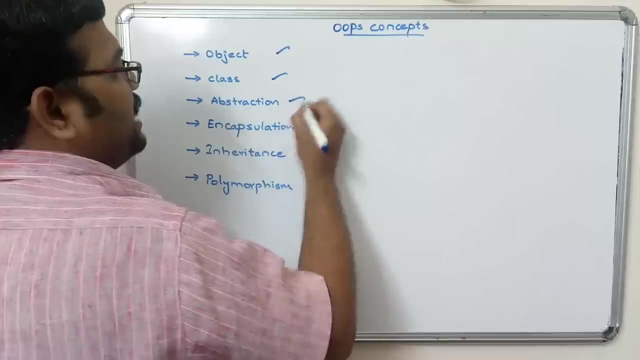 So all the implementation details will be hidden. So this type of applications can be done in java programming that we call it as an abstraction or a data hiding. So I hope you understood this abstraction. Next one: So object class abstraction, Now encapsulation. 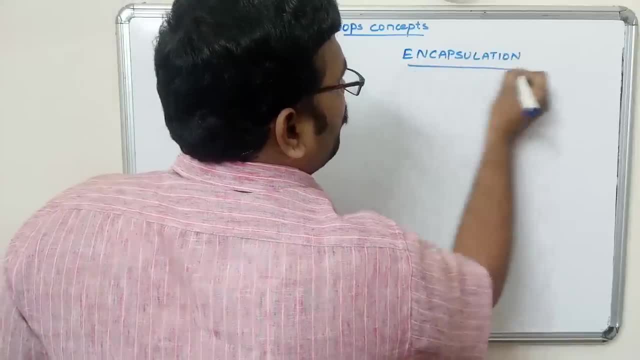 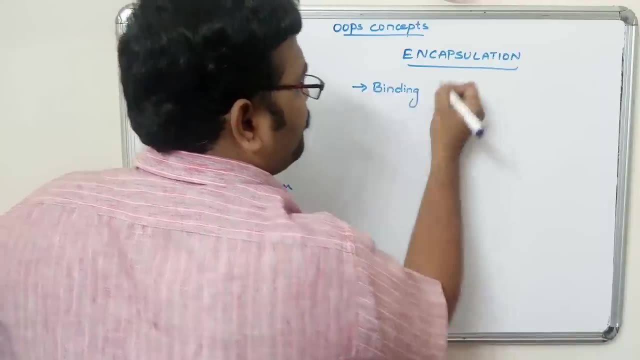 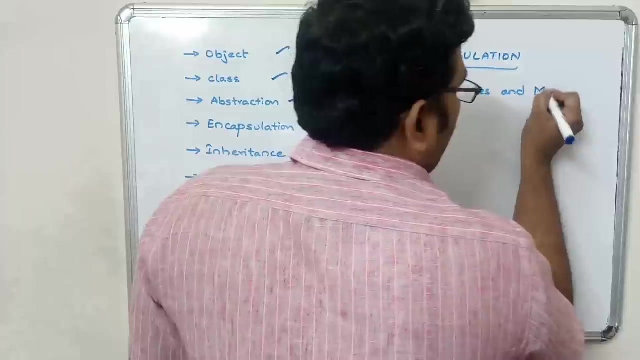 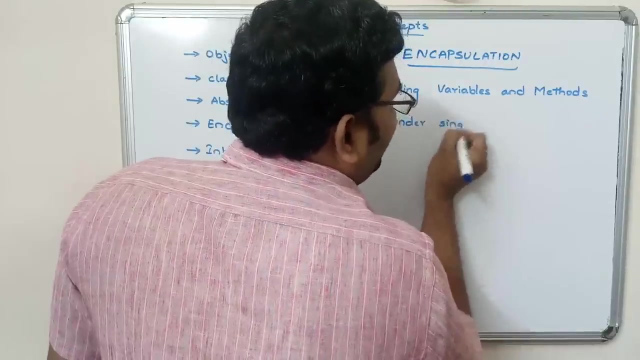 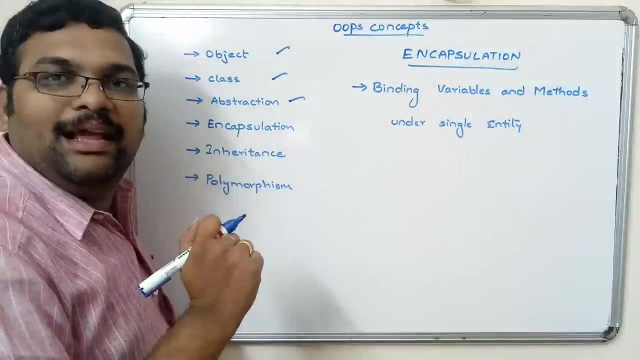 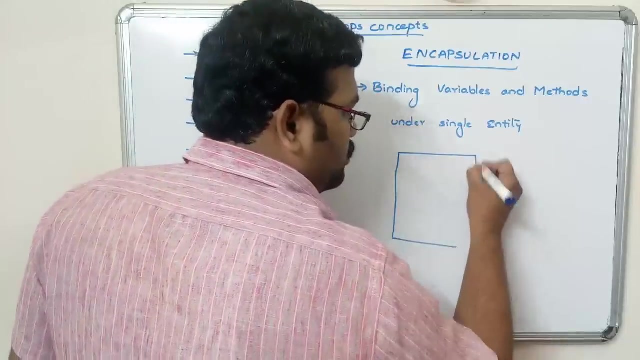 Encapsulation. So this means binding variables and the methods under single entity. Binding the variables and the methods under single entity. Binding the variables and the methods under single entity. So see for understanding. I will write here. So a class is having three parts. One is the name of a class. 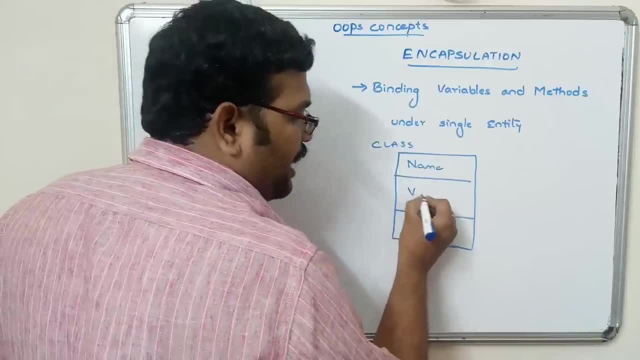 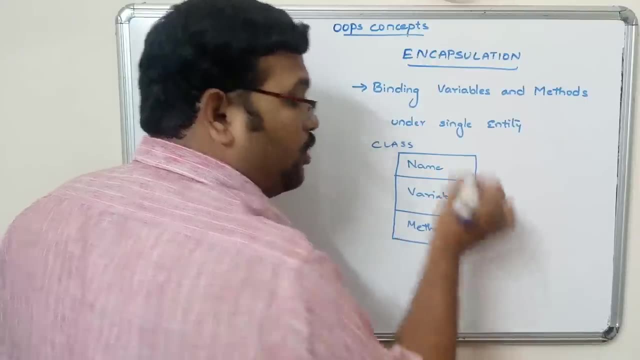 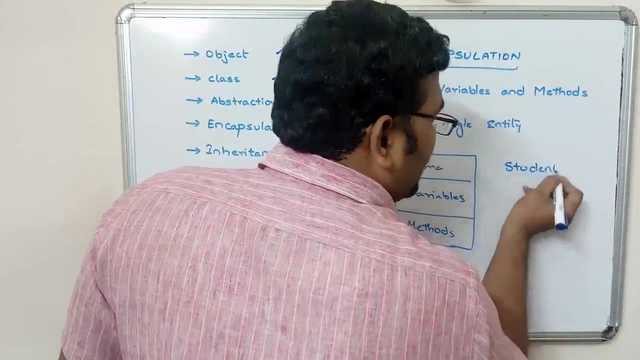 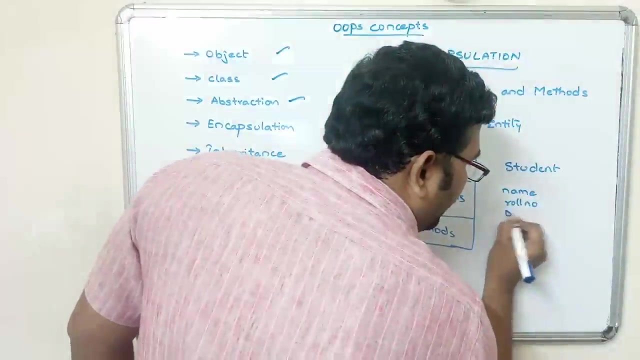 So this is a class. Here we will write the variables And here we will write the methods. Similarly, object is also having the name of a class. Here we will write the name, variables and methods. Simply we can say: student is a class having the variables name, role, number and a date of joining. 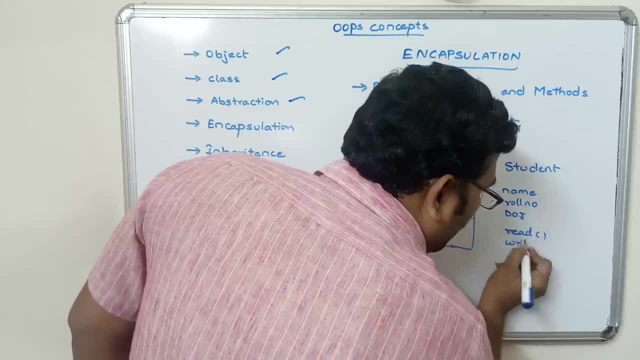 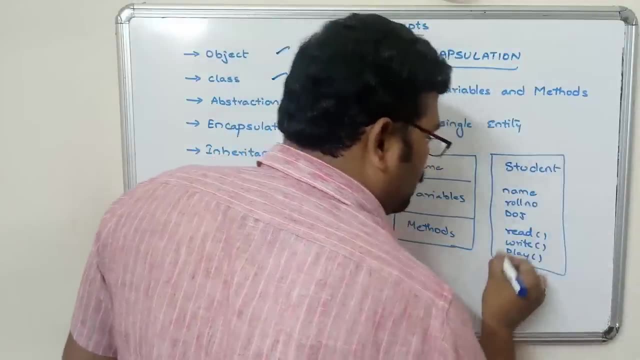 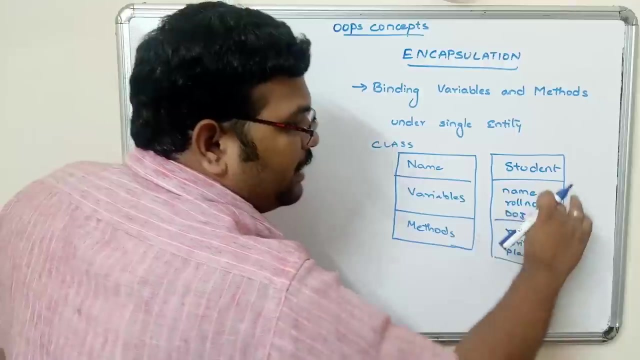 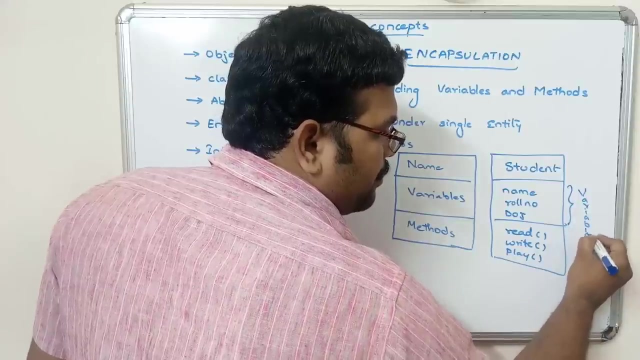 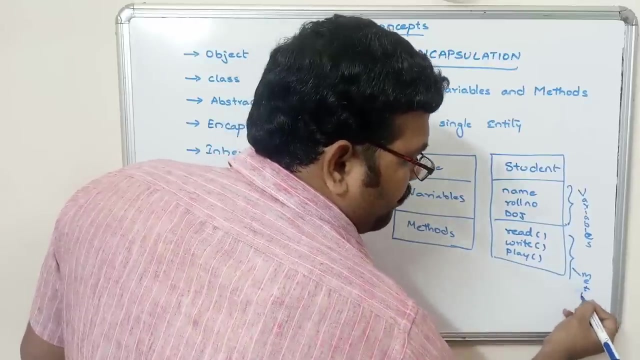 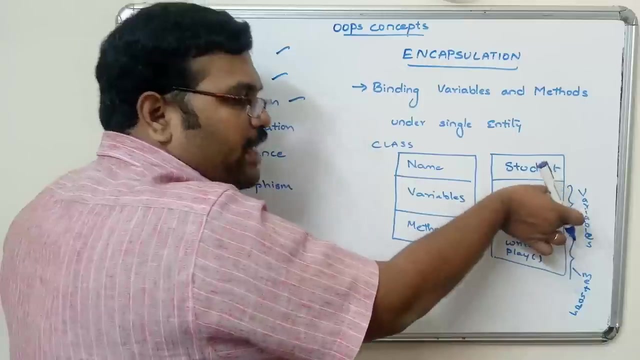 And the methods read, write and play, Right. So this is a class. So here we are writing the variables and these are called variables And this we call as methods. Right, These are called variables, These are called methods. So here we are binding these variables and methods in a single entity. 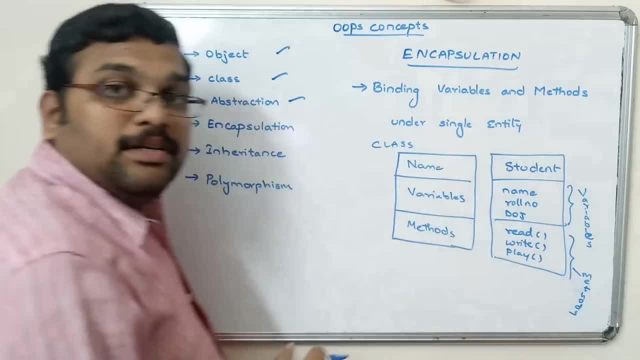 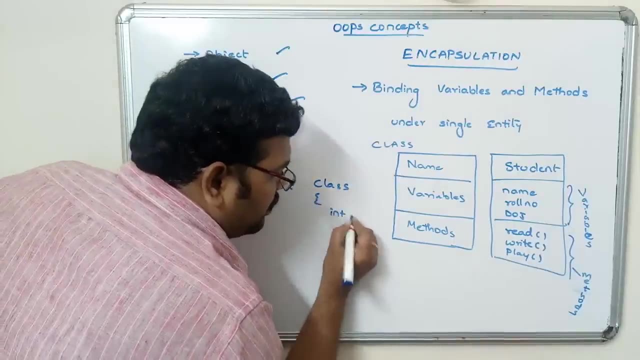 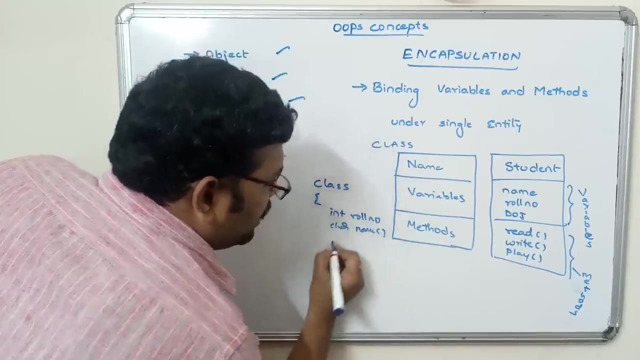 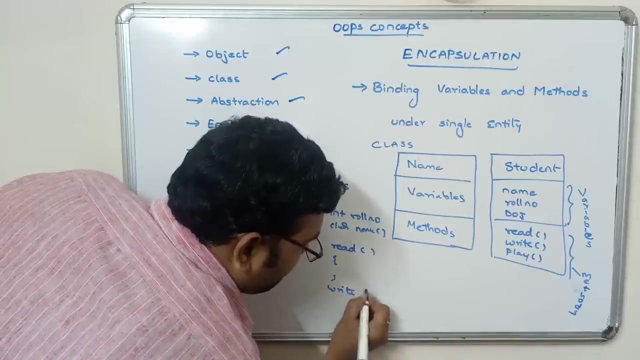 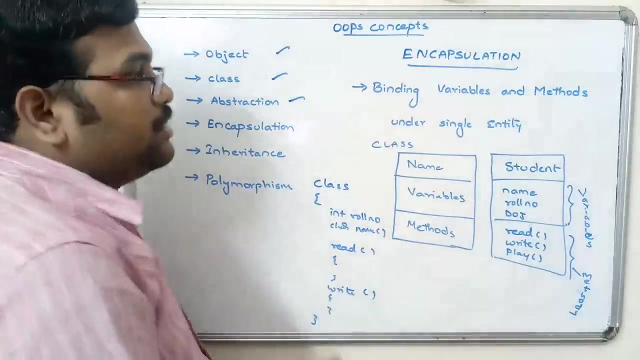 We call it as class or object. So object is also having the same structure. That means one class will be having int, role, number, character, name and similarly read method, write method. So one class consists of variables and methods, Right, So this is called encapsulation. 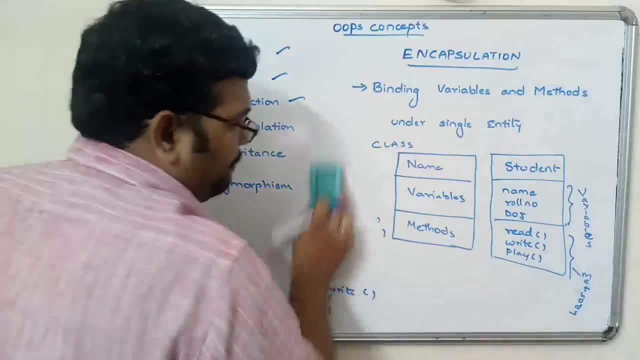 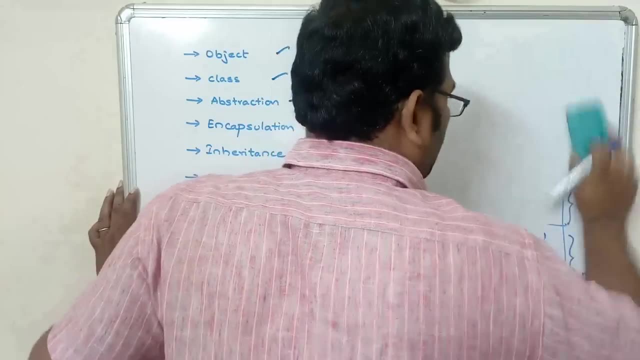 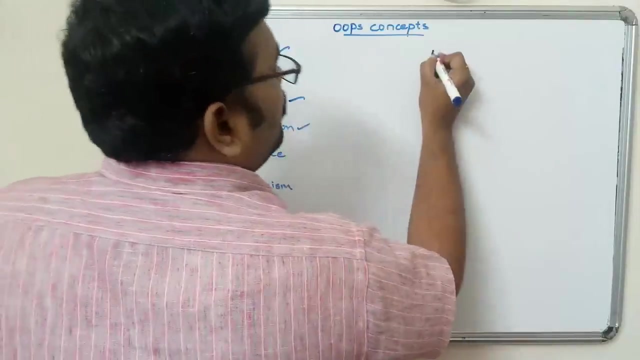 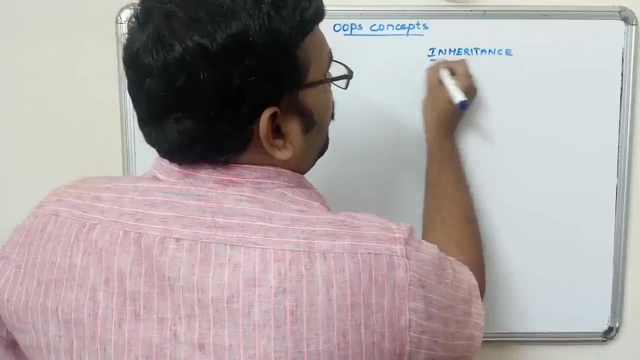 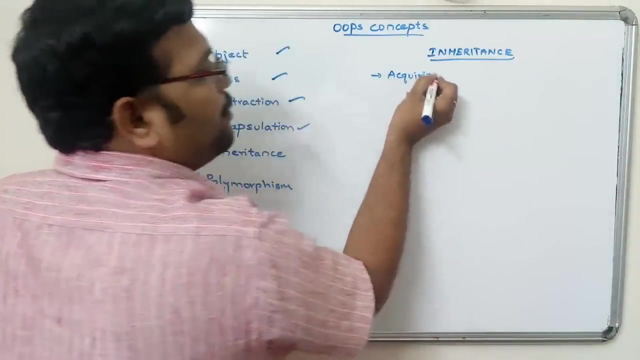 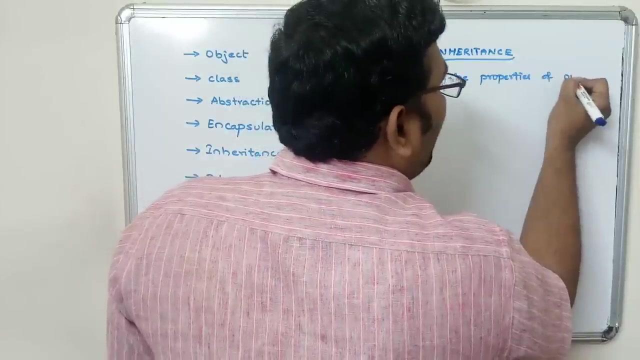 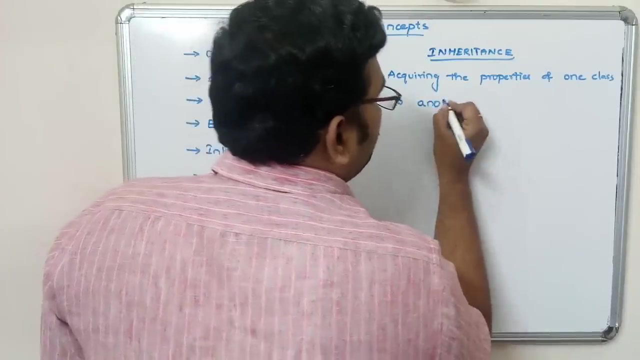 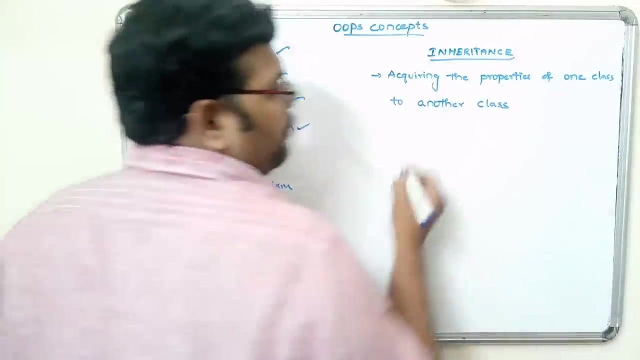 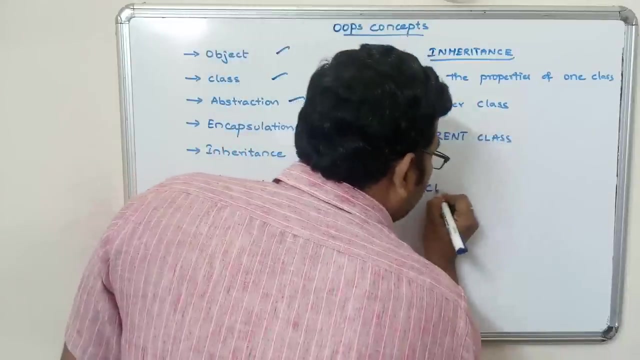 So hope you understood this one. Next, Coming to the next concept: Inheritance. Inheritance. So what is meant by inheritance? Acquiring the properties of one class to another class, Acquiring the properties of one class to another class. Simply, we can say it as parent class and a child class. 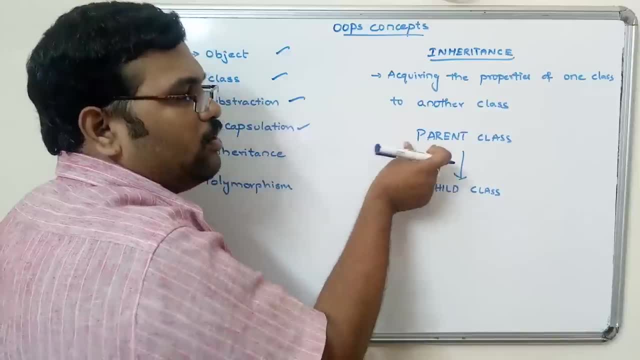 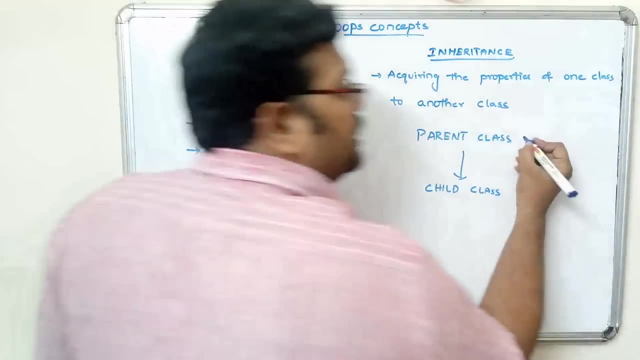 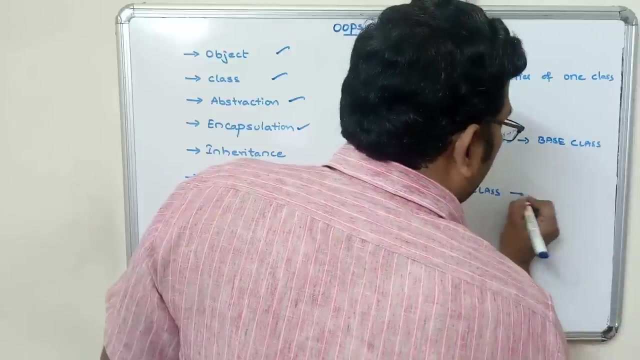 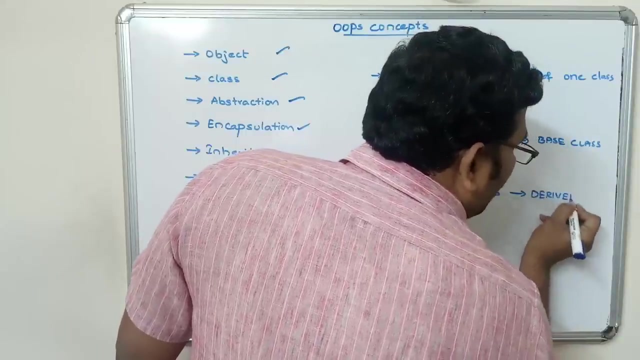 So child class will acquire the properties of parent class. Right Child class will be having acquiring the properties of parent class. So this we call it as base class Or we can call it. this child class will be called as derived. So a derived class is a class which is derived from the base class. 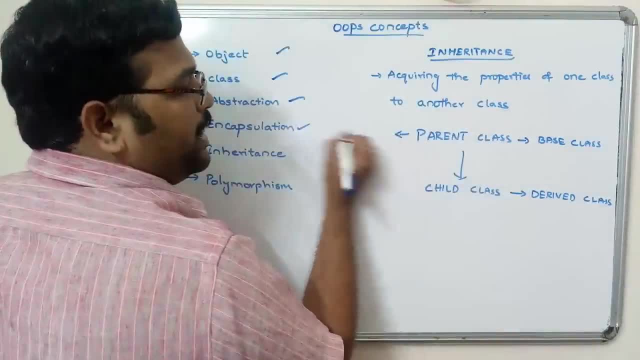 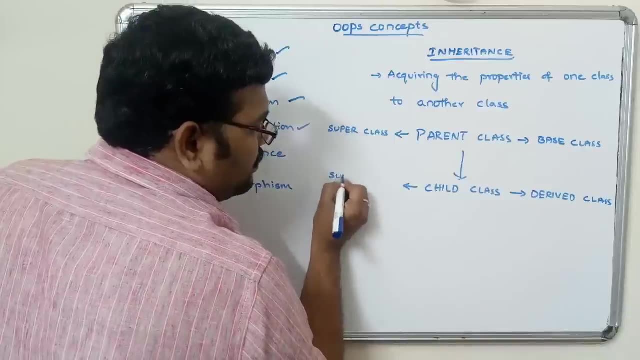 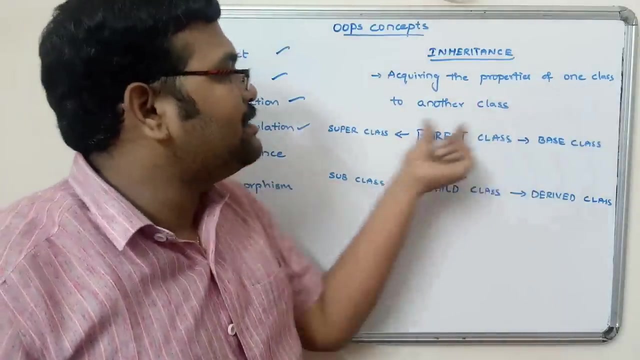 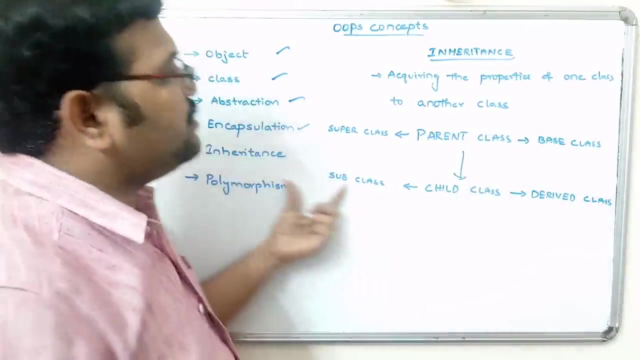 Derived class. Or we can call this parent as super class And this child class as subclass Right, So acquiring the properties of one class to another class, So here acquiring the properties of parent class to the child class. So this concept, we call it as inheritance. 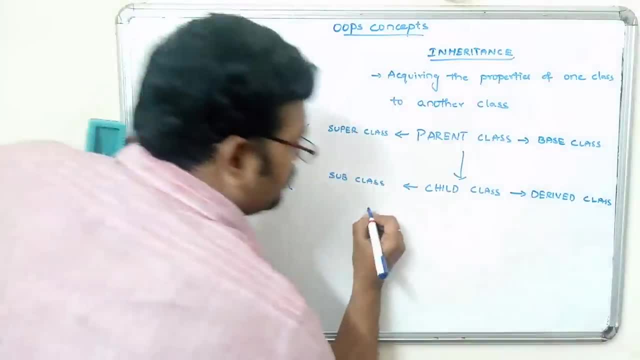 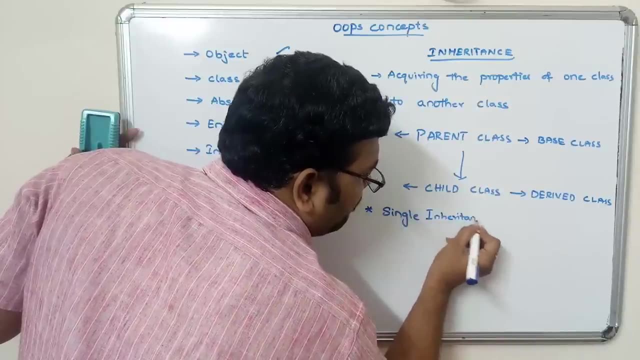 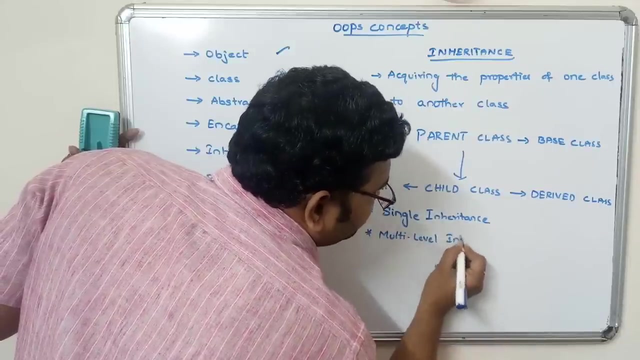 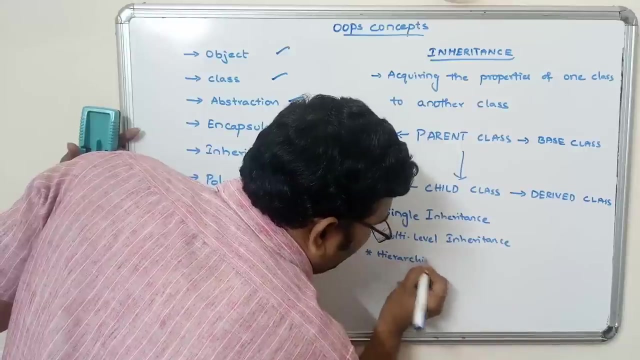 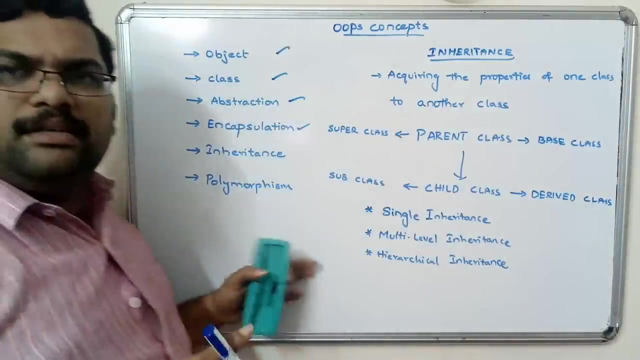 So here there are different types of inheritance: Right, So we will have a single inheritance, Multi level inheritance And hierarchical inheritance. So let us see the basic introduction. Then we will move on by one by one Right, So we will see one by one concept in the depth. 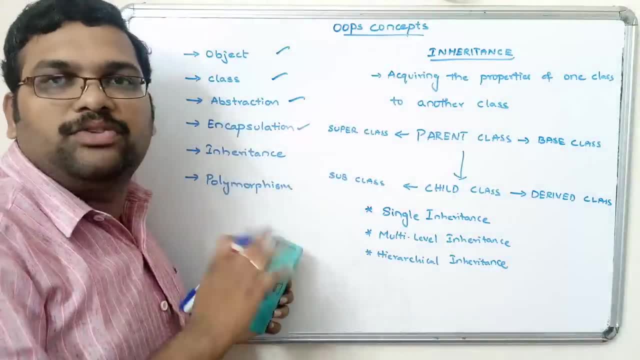 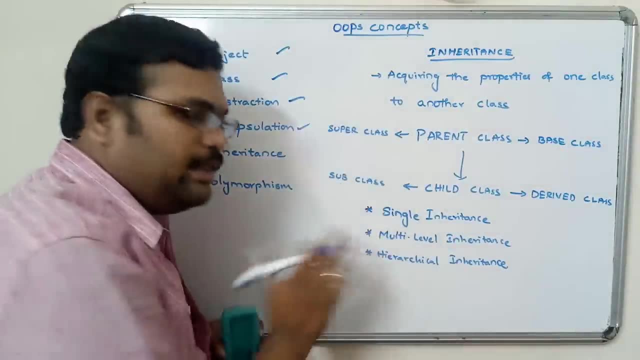 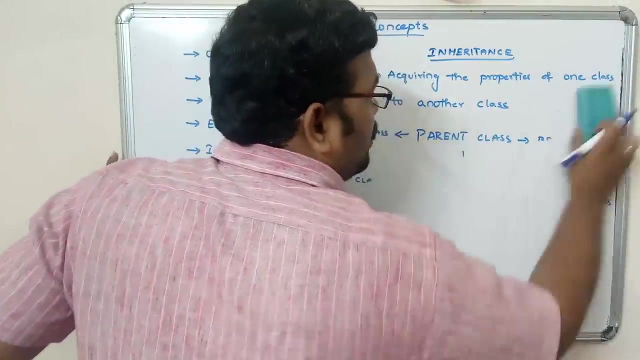 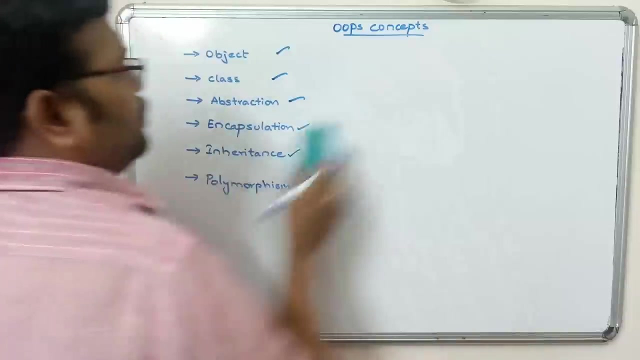 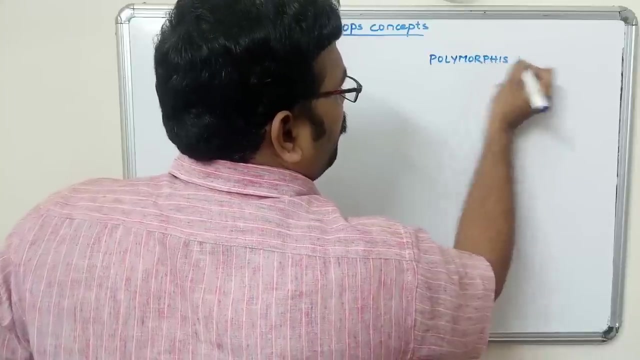 Now in this session, let us cover the introduction of all these object oriented concepts, So we can have these three types of inheritance: Single inheritance, Multi level And hierarchical. So this is called inheritance concept. Next, Coming to the polymorphism, So performing the same task. 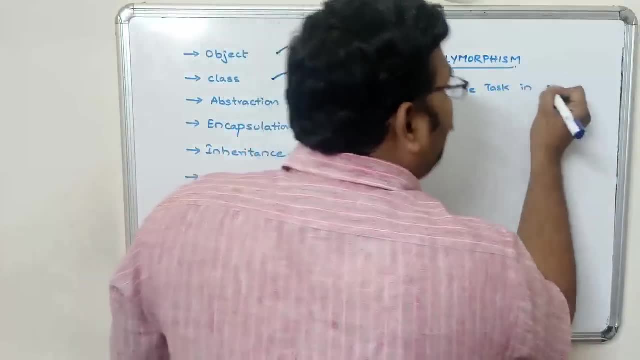 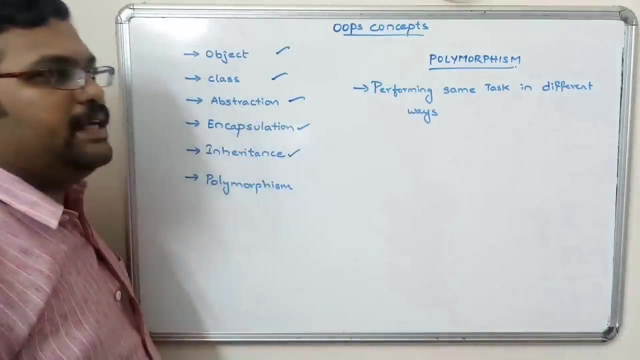 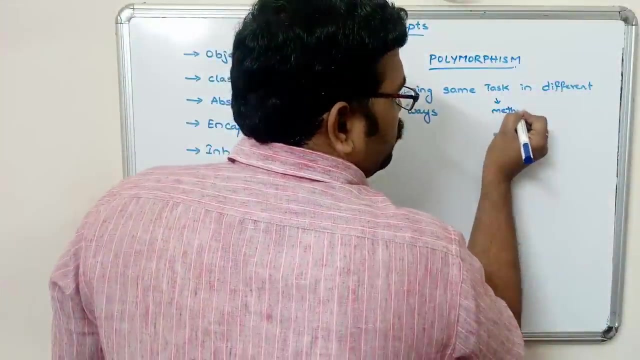 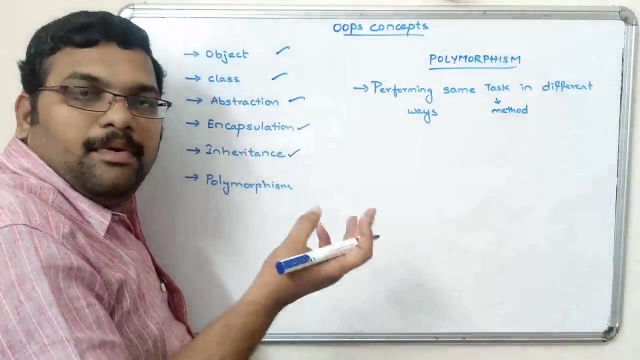 Same task In different ways, In different ways. That is called as a polymorphism. Here task means a method, Method, So invoking the method in different ways. For example, If we are having a program For adding of two numbers, 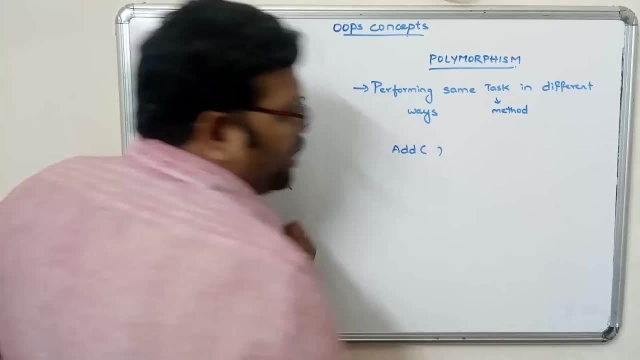 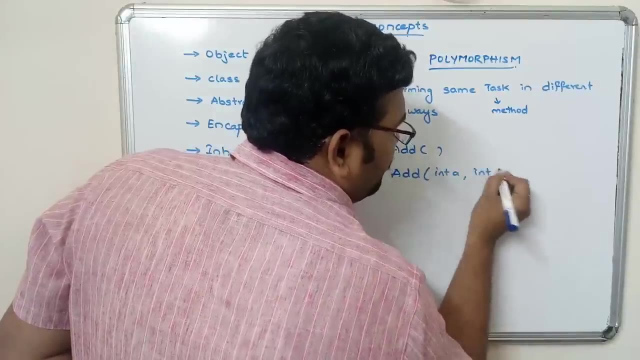 We can write Add Simply. we can call add Without any parameters. We can call Add with int a comma, int b Right. So two methods. So both will perform the same task, But implementation is different. Here we are not passing any arguments. 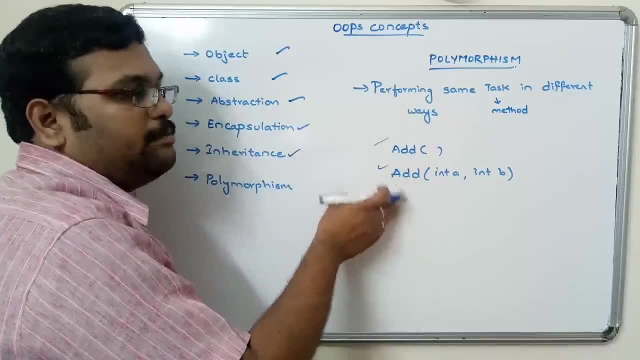 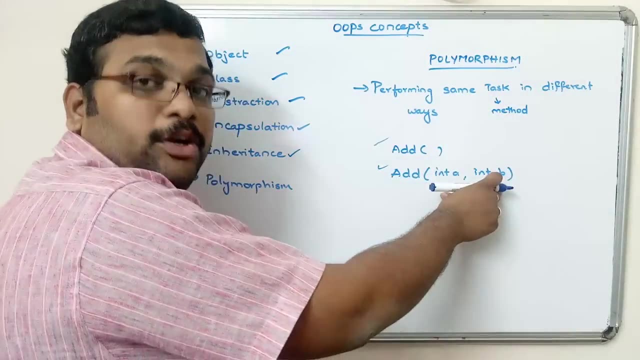 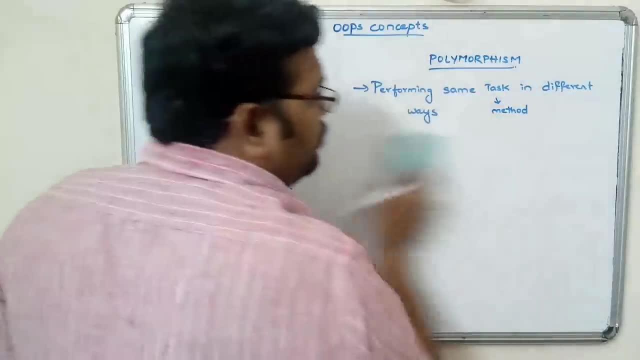 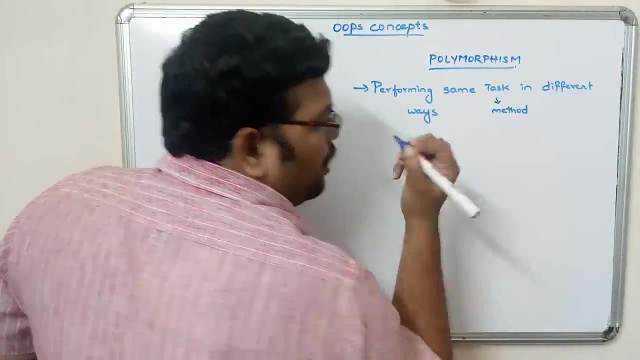 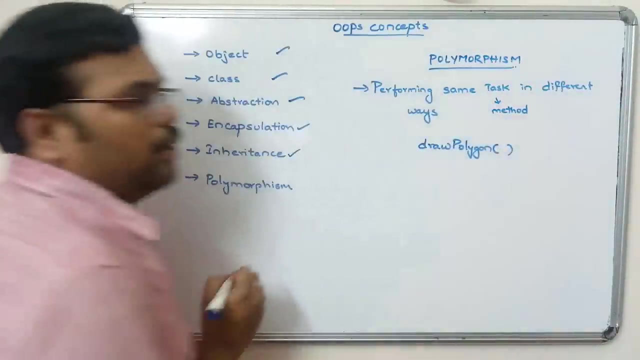 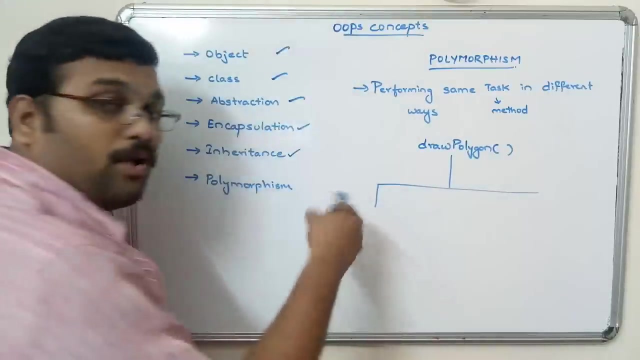 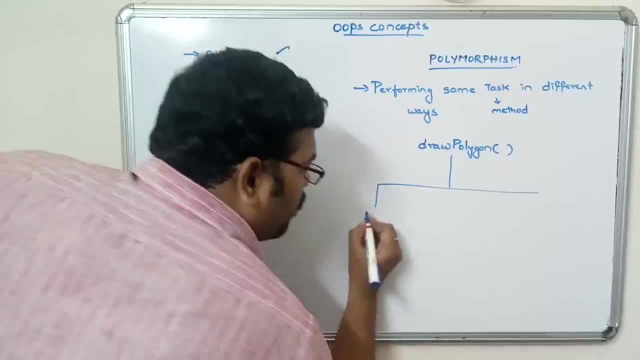 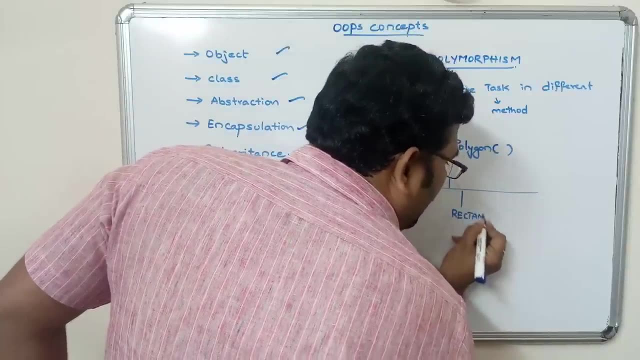 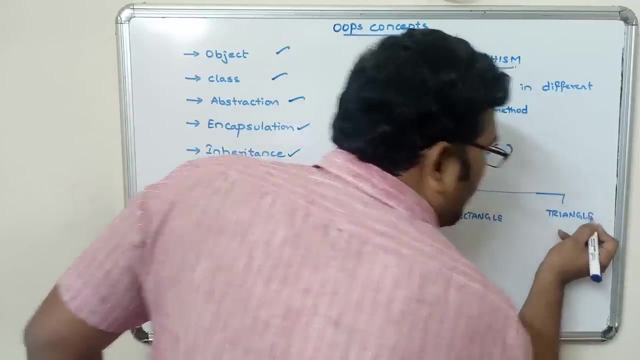 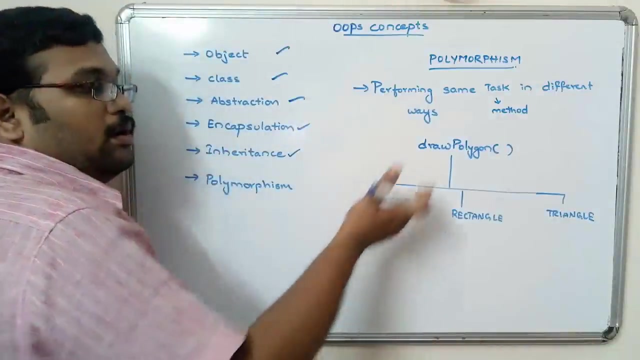